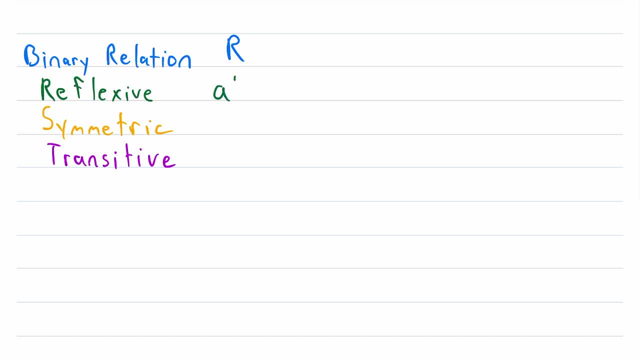 R. R is a reflexive relation if every object under consideration relates to itself. For example, equal to is an equivalence relation and for is equal to itself. So that's an example of the reflexive property. Again, our relation R is reflexive if every object under consideration. 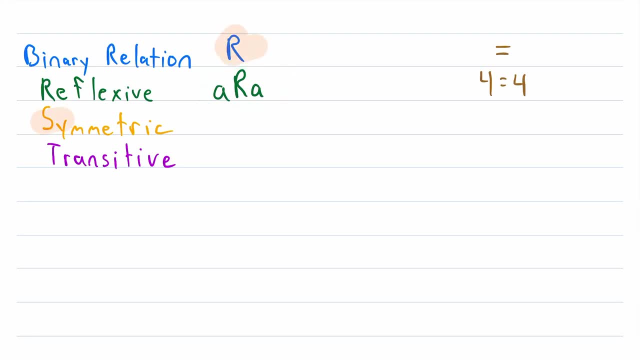 relates to itself. Next, the relation R is symmetric if A relating to B implies that B relates to A. So, for example, if an object under consideration relates to itself, for R to be symmetric, this has to be true for all objects under consideration Anytime. object 1: 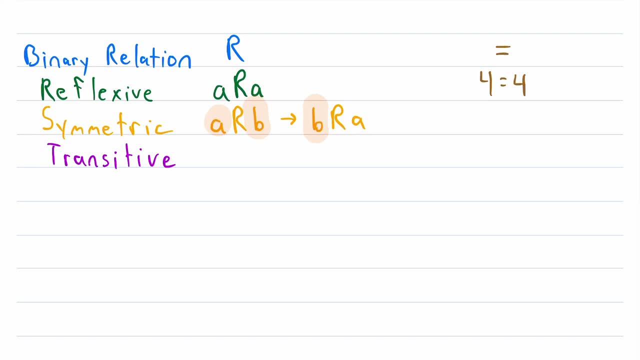 relates to object 2, object 2 must also relate to object 1.. That is what makes R a symmetric relation, For example, with the relation equals, 3 squared is equal to 9.. And it is also true that 9 is equal to 3 squared Equal to is a symmetric relation. The last property that R has to have. 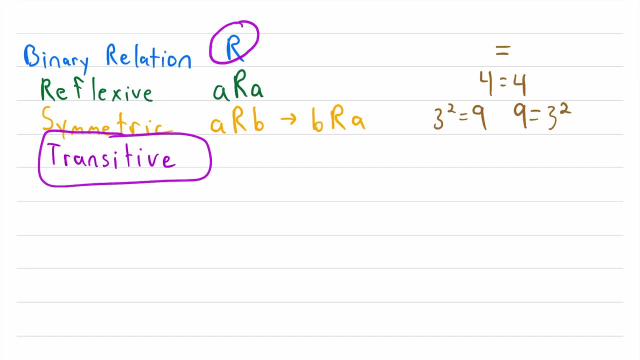 in order to be an equivalence relation, is that it has to be transitive. We say that R is transitive if, every time an object A relates to an object B and the object B relates to an object C, it is also true that A relates to C. 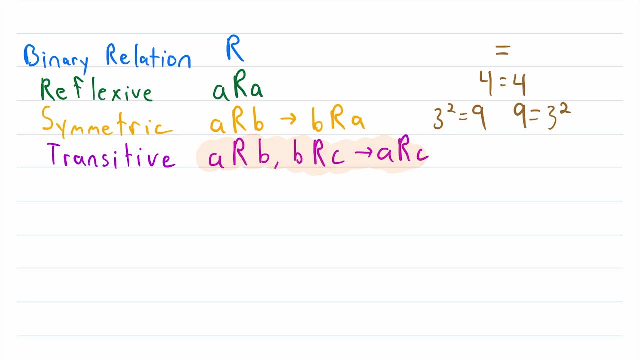 And again, this has to be true for all objects under consideration. If there are three objects- A, B and C- such that A relates to B and B relates to C, then it must also be true that A relates to C in order for the relation to be true for all objects under consideration. 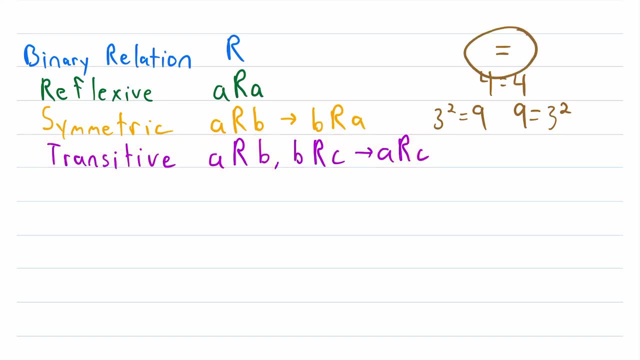 As an example of this with our equals relation, 2 is equal to the square root of 4, and the square root of 4 is equal to 4 divided by 2.. And it is also true that 2 is equal to 4. 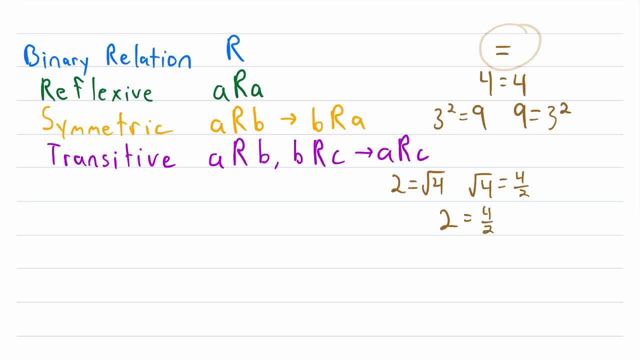 divided by 2.. Equals is a transitive relation. So since equals or equal to is a binary relation that is reflexive, symmetric and transitive, it is an equivalence relation. Can you think of a relation that is transitive? If you think of a relation that is transitive, it is an equivalence relation.